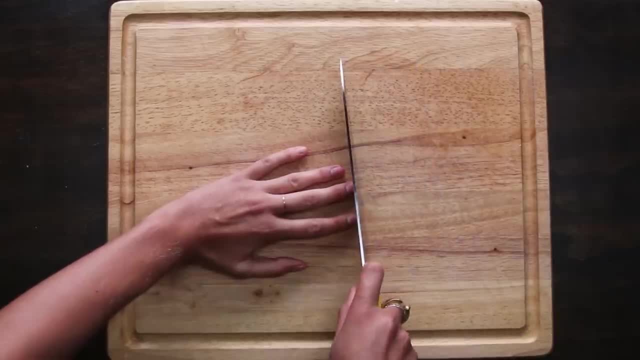 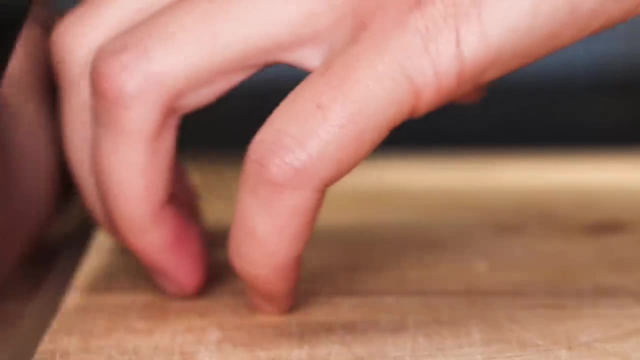 As you can see, my fingers are in danger of getting cut off. You actually want to form a claw so that your fingers go in and the knife will hit up against your knuckles as you're chopping. So with this claw, your fingertips are going to be protected the whole time. 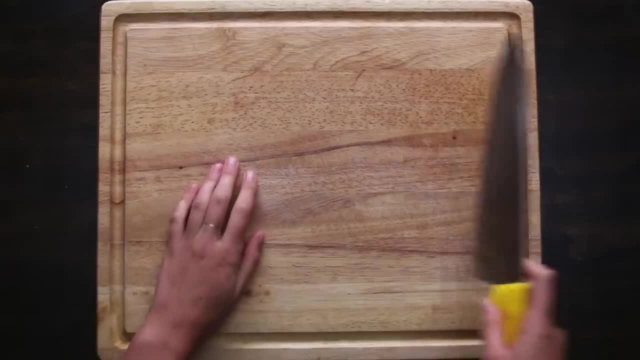 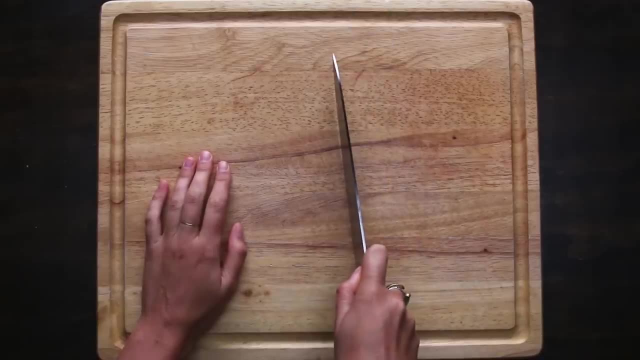 and it's actually going to give you support as you're chopping. Another common mistake is the slicing motion. If you just chop really aggressively down like this, you're not going to get a nice cut. You really want to do a rocking motion when you cut, going back and forth with the knife. 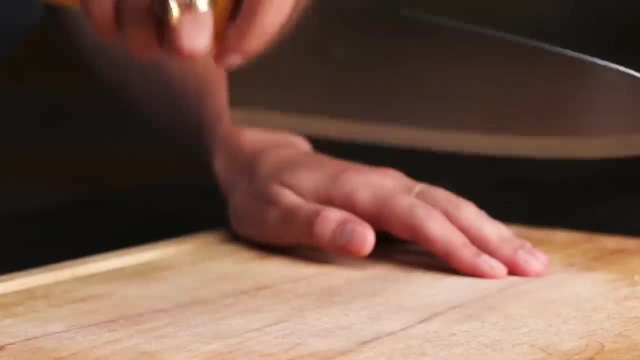 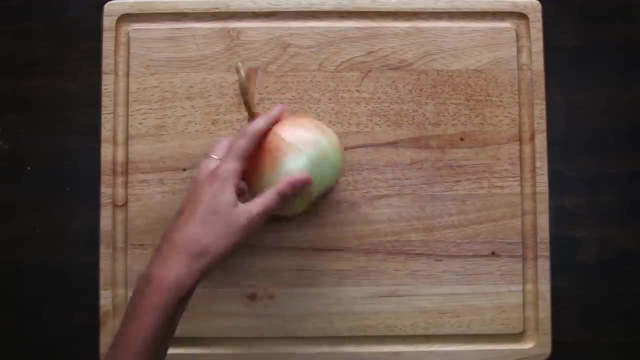 Think about it like a wave. So now that you know how to hold a knife properly, we're going to demonstrate a few common cuts that you see in recipes. We're going to start out with a dice, So for an onion, which is probably the most common thing, you're going to dice. 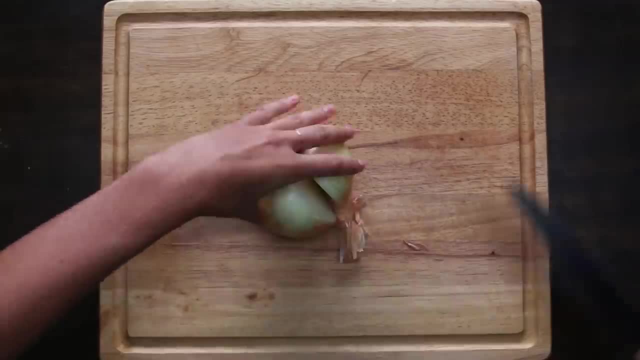 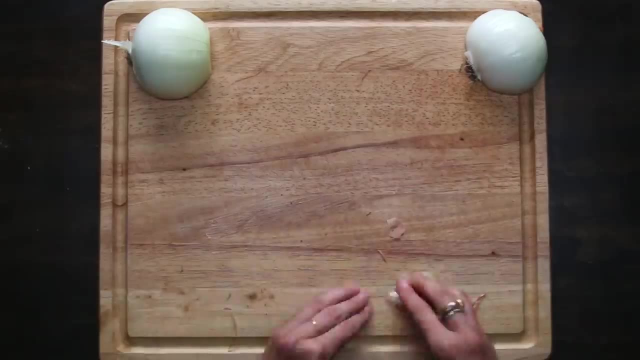 you want to cut it in half first, right through the root end. So the next step is to peel the outer layers, making sure that the root end is still intact. So with dicing you want to make sure that the flat side is down, so it'll give you the most stability. 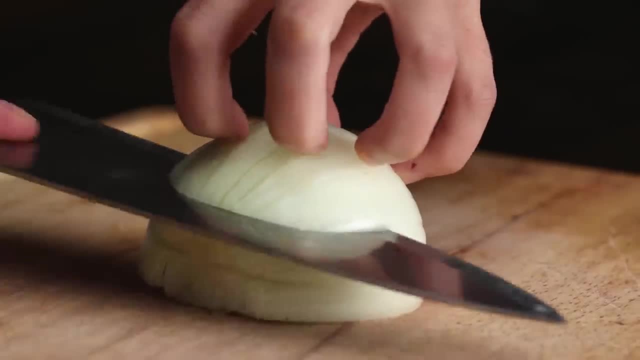 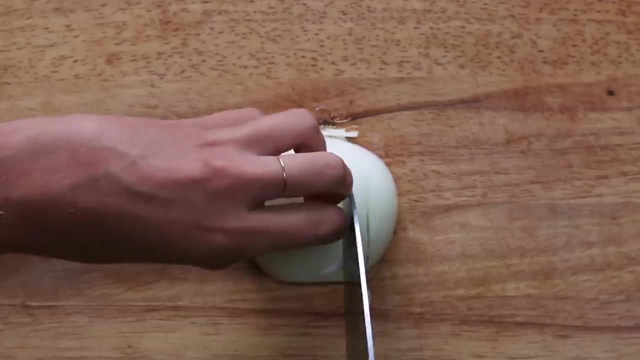 Making sure we have that claw grip. make a few incisions horizontally into the onion- then you're going to turn the onion towards you with the root side furthest away- and again with that claw, make a few cuts vertically, Turn the onion again and use. 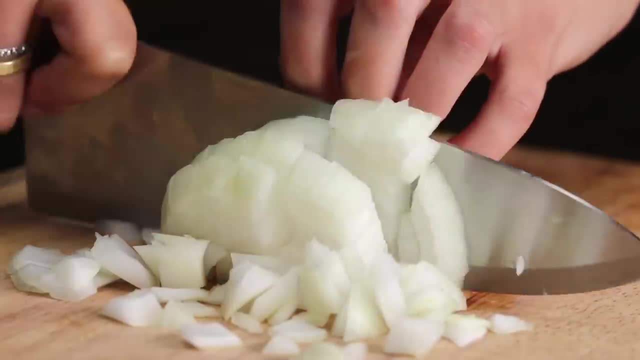 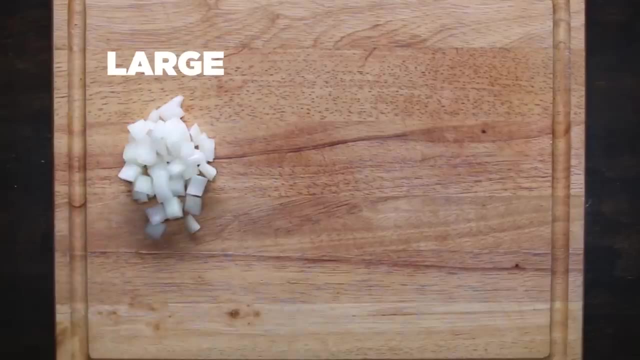 your knuckles as a guide and you're going to start chopping along and just do that same nice chopping, wave, motion down, And then look, you've got an even dice. This is an example of a large dice. Here we've got a medium dice, and over here we've got a small. 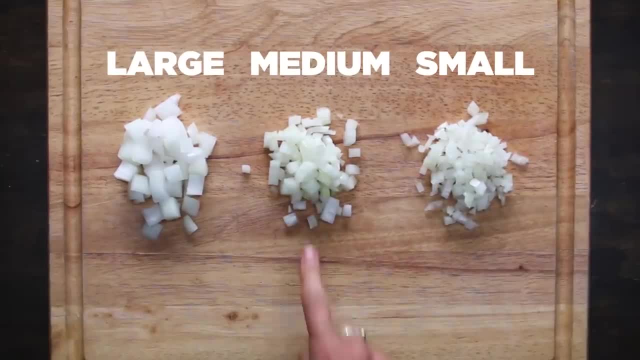 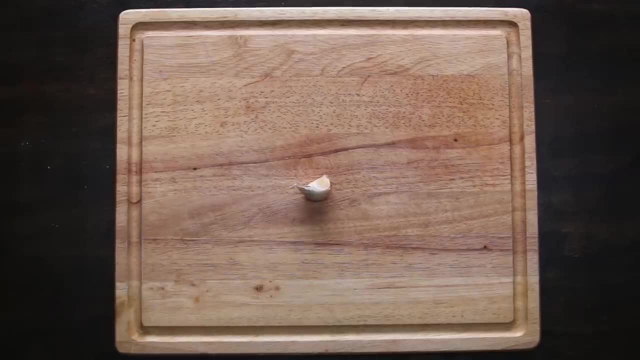 dice. So in most recipes, when you just see something that says dice, it should be a medium size. The next cut we're going to show you is mincing. The most common of these is minced garlic. You want to remove the root end and again. 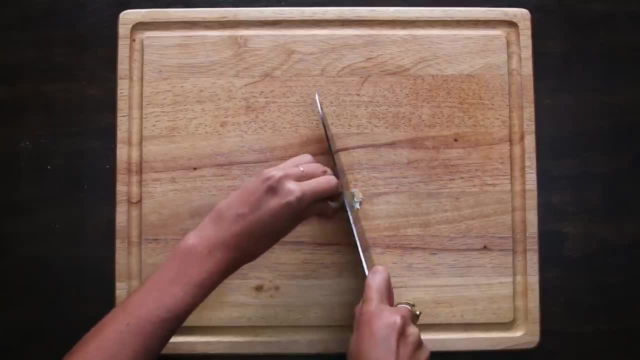 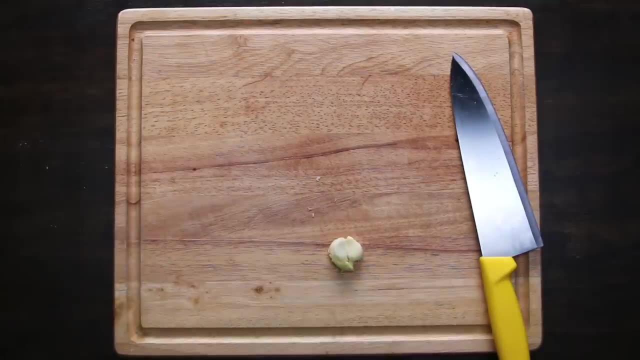 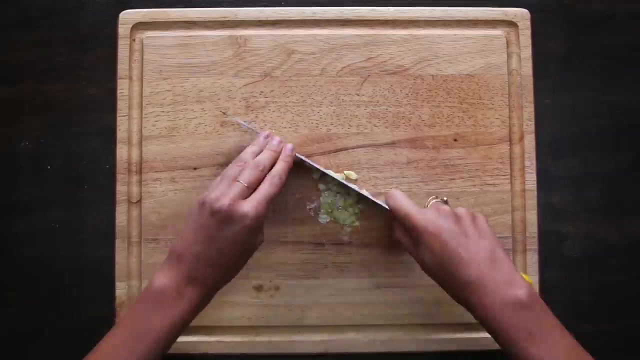 remember, we're always using that little claw. The next step is to place the garlic under the blade and then smash down. Then you're gonna peel the garlic- The papery skin should fall right off- and then again use that claw, use that same wave motion, and you're just going to repeat this a ton of times. I mean you. 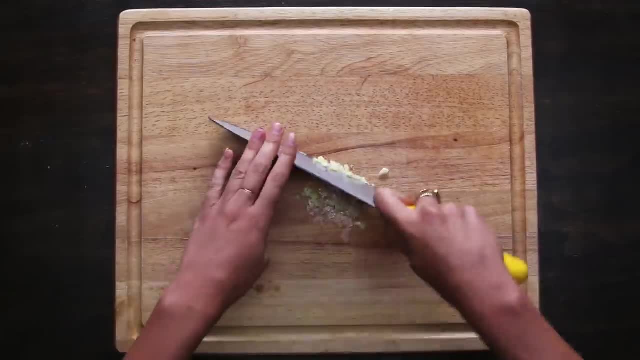 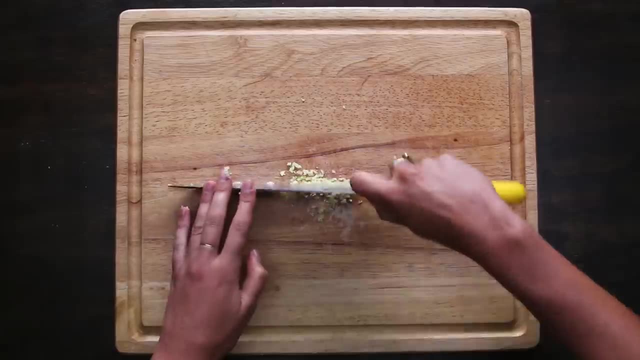 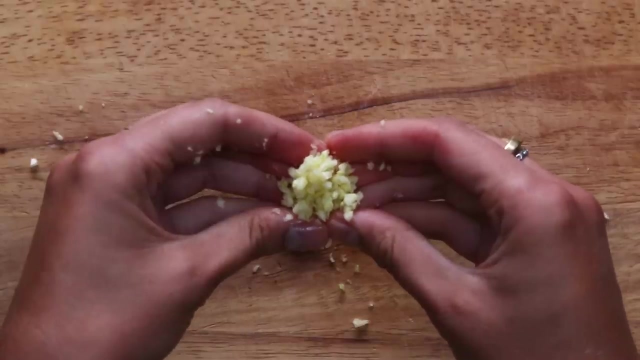 can use your fingers on the other side of the blade to help stabilize you and then gently scrape it off With mincing. the finer the mince, the more flavorful your dish is gonna be, and it should really be tiny. Anything bigger than this would be a fine chop, Similar to dicing. mincing is a really common cut You can. 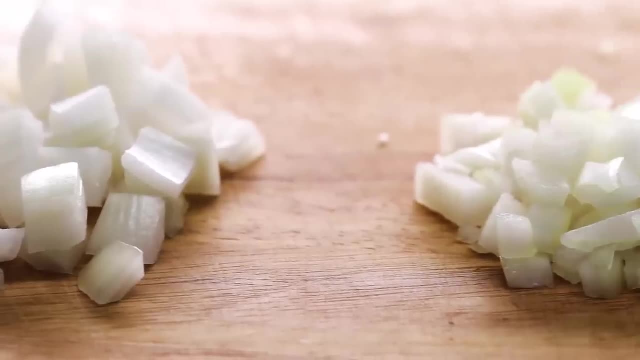 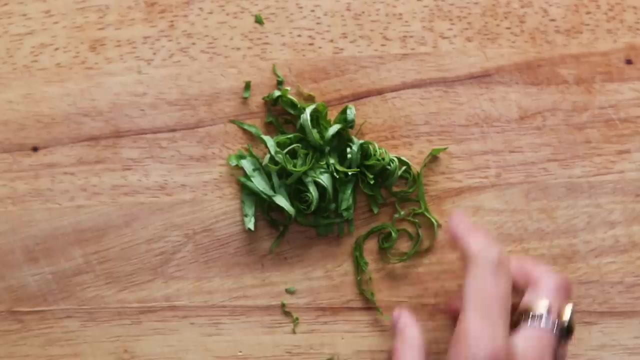 use it in so many preparations. So dicing and mincing are the most common cuts you'll see in recipes. but we're gonna show you a few other cuts and in case you want to get fancy, Next up is chiffonade, which is most commonly used. 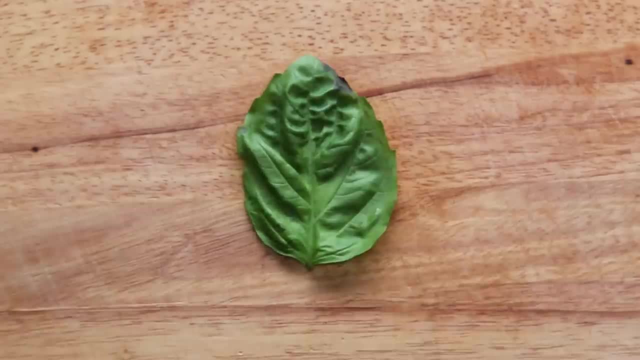 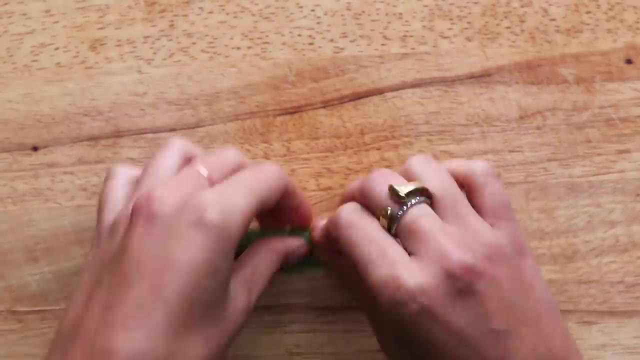 with herbs. We're gonna show you with some basil. So first you're gonna stack basil leaves in a pile, then you're gonna roll them up from the top all the way down in a really tight cigar shape, So it looks like that, and then again not to. 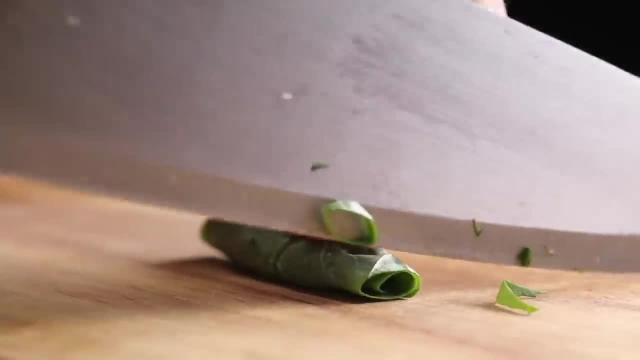 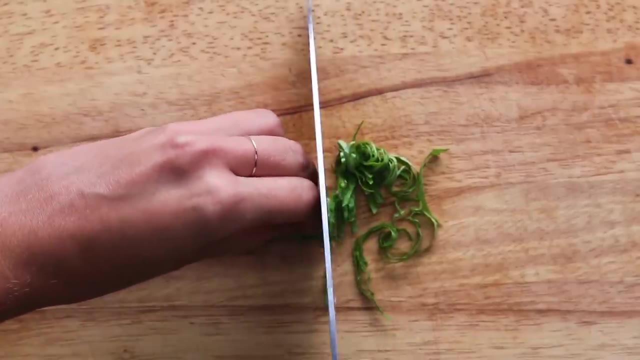 sound redundant, but you're going to use that same motion and just do really, really thin slices. A common mistake when you're doing the chiffonade cut is to not use enough force. You want to make sure to fully slice down and if you do it correctly, it should look like these: 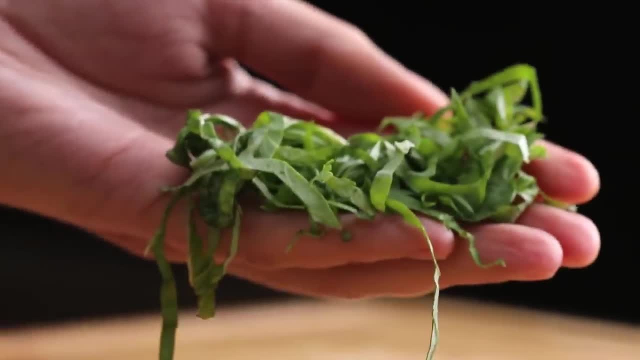 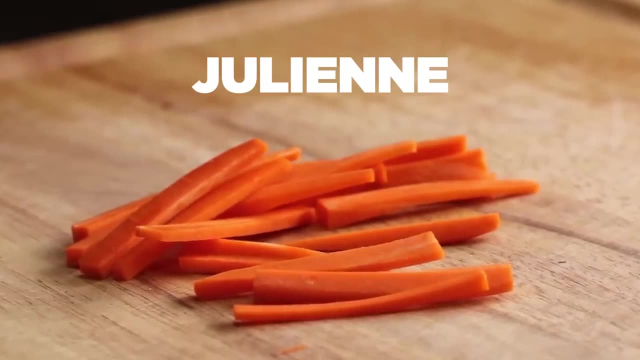 beautiful ribbons. The chiffonade is a really pretty cut, but it's really a vanity cut. You typically use it to garnish dishes. The next cut we're gonna show you is julienne, which is most commonly used with carrots. but you can. 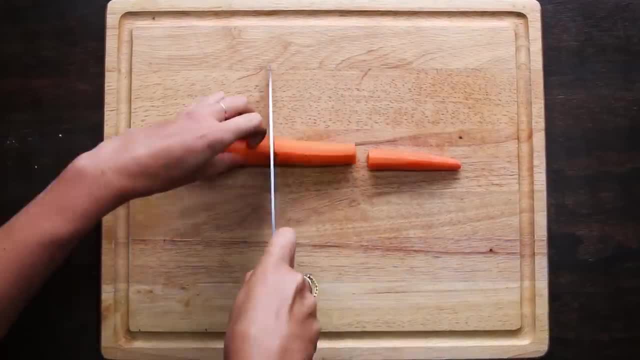 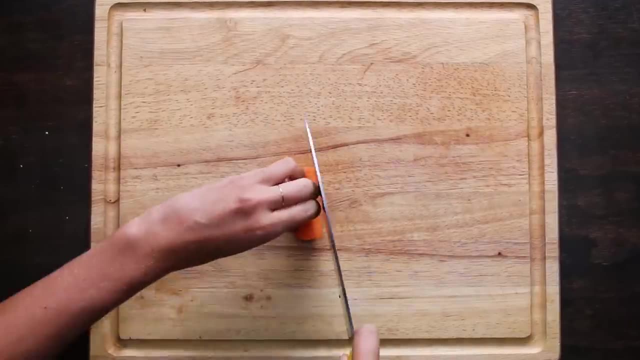 do it with all sorts of things. So, to julienne a carrot, you want to cut it into about two inch segments. We're gonna just start with one for now, To start. you want to create a flat base. Once you've cut that flat part off, put the flat part. 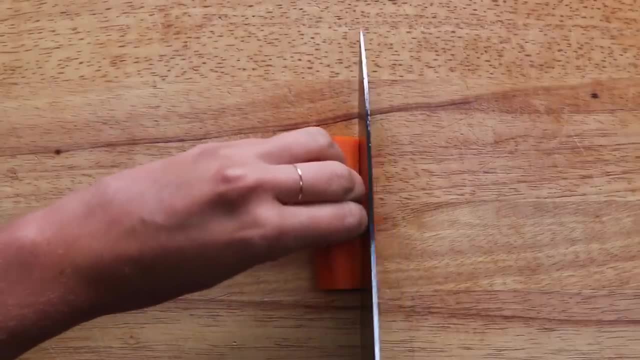 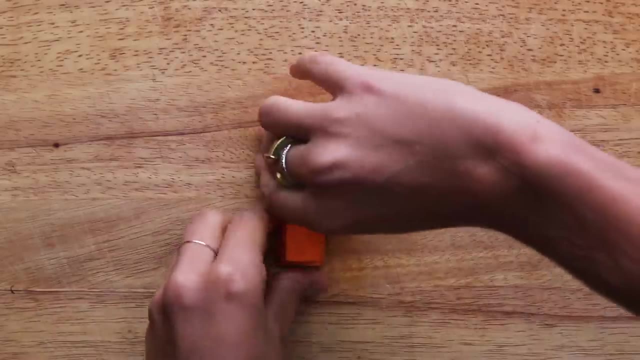 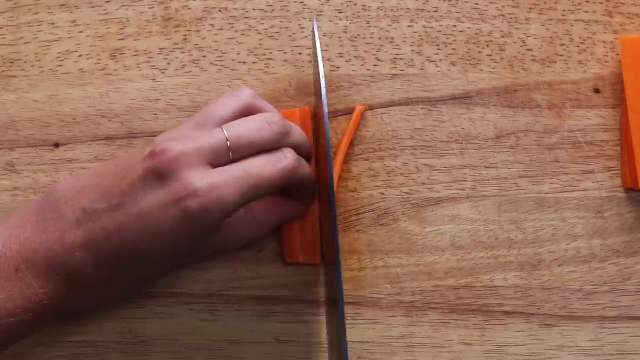 on the cutting board so you have more stability. Then I want to make 1 eighth inch equal slices down. Next, stack the carrots up like building blocks. You can also divide the carrot stacks up into two parts, so it's a little easier to manage. and then again you're gonna want to make equal 1 eighth of an inch slices. 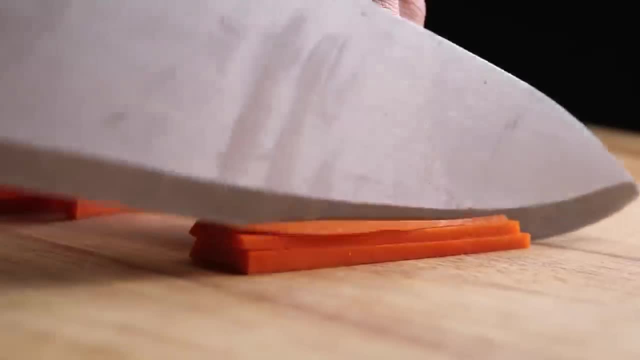 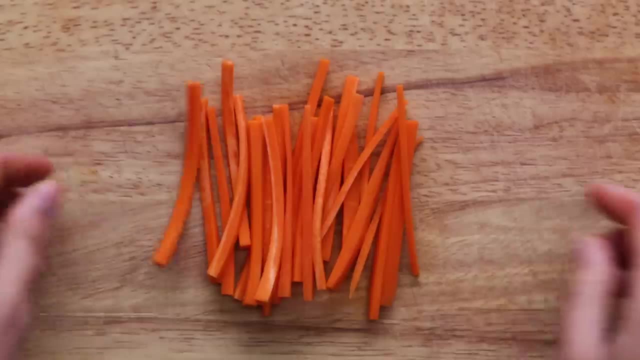 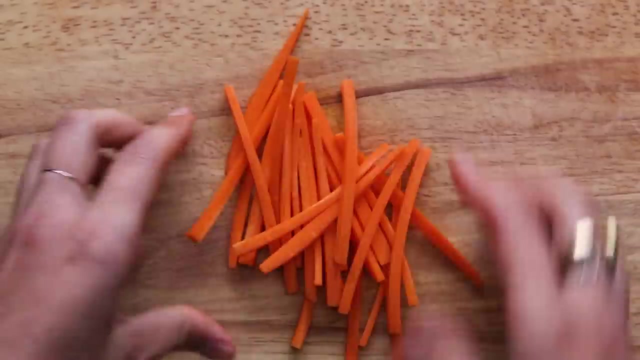 down and then you should get these beautiful, equally sized matchsticks. Julianning is not a super common cut. You primarily see it in raw preparation like something like a quick pickle. It's really great, because you wouldn't want a huge bite of pickled carrot, but with a julienne or a matchstick it's just the.